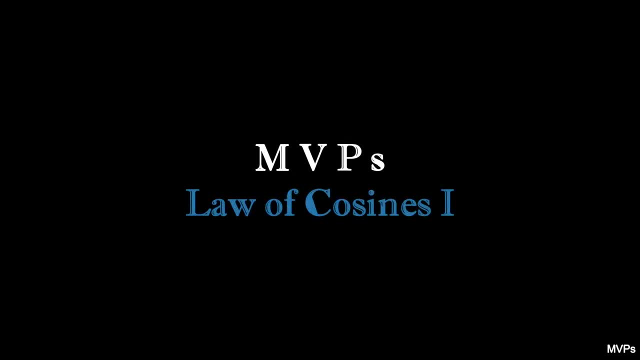 Consider a triangle with sides of length A, B and C and angle theta opposite to C. Draw the circle containing the triangle using the side length of A as the radius. Extend the radius to a full diameter and extend the side length C to a diameter by. 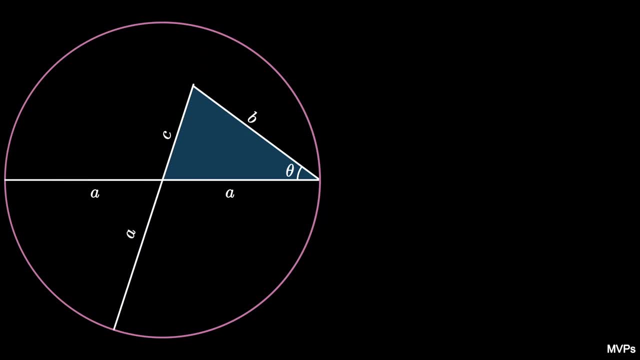 connecting a radius of length A and a segment of length A minus C. Extending the side length B to the circle and connecting that line to the other end of the horizontal diameter results in a right triangle according to Thaley's Triangle Theorem. 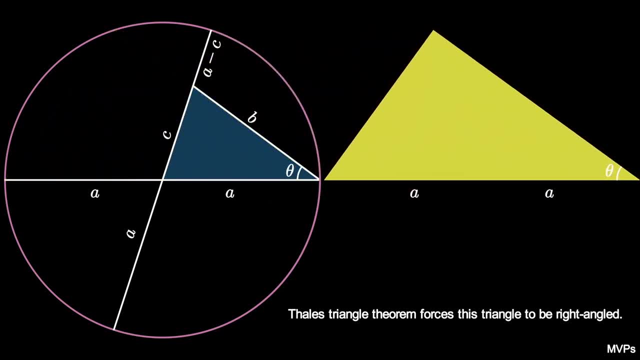 This right triangle has a hypotenuse of length C. It has a length 2 times A. This means that the leg adjacent to the angle theta has length 2A cosine of theta. Therefore, the line segment extending the length B to the circle has length 2A cosine. 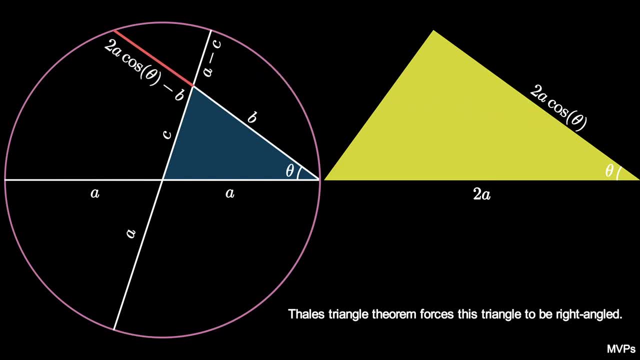 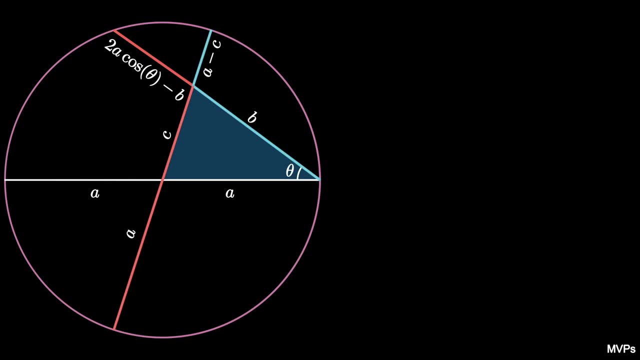 theta minus B. Now we have two intersecting chords in the circle. So by the Intersecting Chords Theorem we have two intersecting chords in the circle. We get that the product of 2A cosine theta minus B times B equals the product A minus. 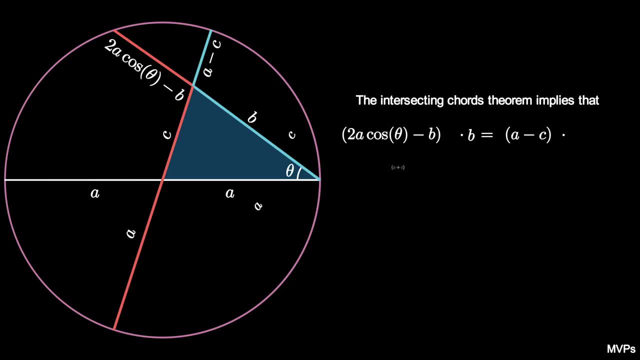 C times A plus C. Expanding both products produces the equality 2A times B. cosine theta minus B squared equals A squared minus C squared. Adding B squared plus C squared to both sides results in 2A times B cosine theta plus C squared. 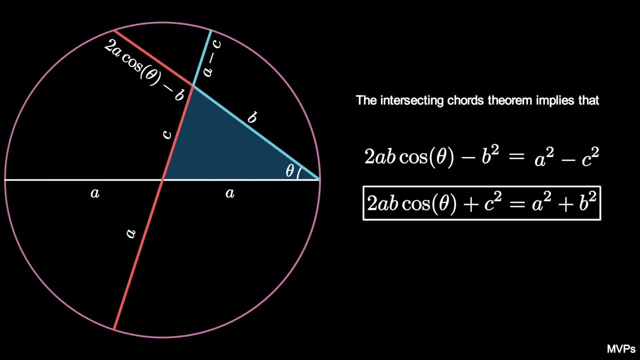 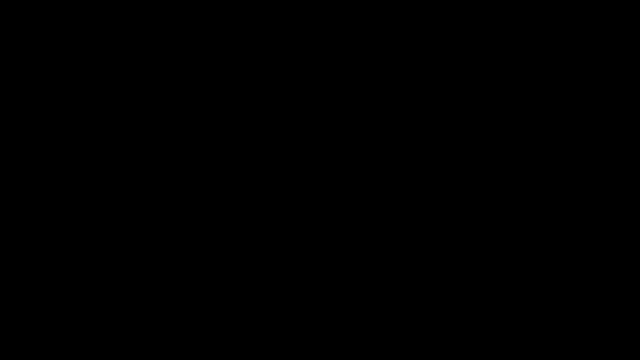